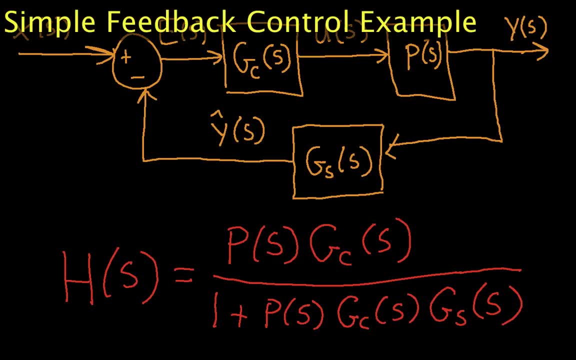 Okay, the purpose of this video is to do a simple example of a feedback control system, mostly so you can get an understanding of the nomenclature in the video in the previous video and also just to give you a feeling for the sorts of things that happen in feedback control systems. 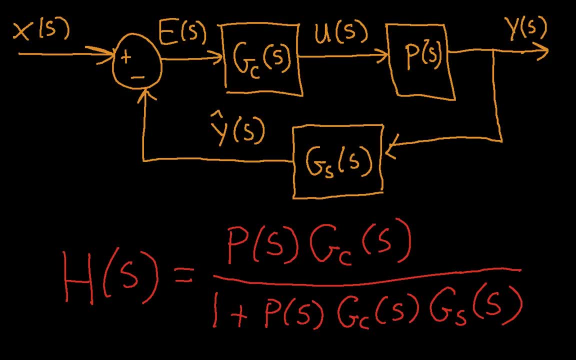 Again, this is going to be a very simple example. Much more complex examples will probably follow. So in the previous video we developed this transfer function, which basically tells us the relationship between the output of this feedback system and the input, And in this video we'll do a much simpler system using these results and show you what we get. 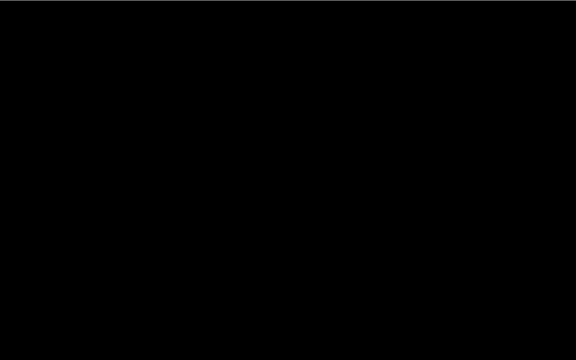 So the simpler system that we're going to do is a simple model do. that we will do is the following: I have a desired input, I compute an error, I'll show exactly what that is in just a minute And I have a simple gain as my controller. 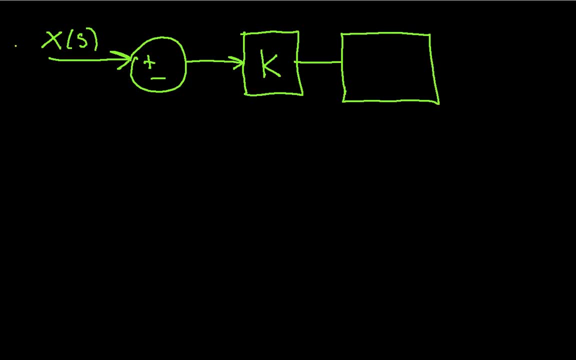 I'll have a plant that basically has a transfer function: 1 over s plus 1.. This is a fairly pedestrian transfer function. It represents something that starts off and grows exponentially until it levels off at some steady state value. We'll have the output fed back directly into. 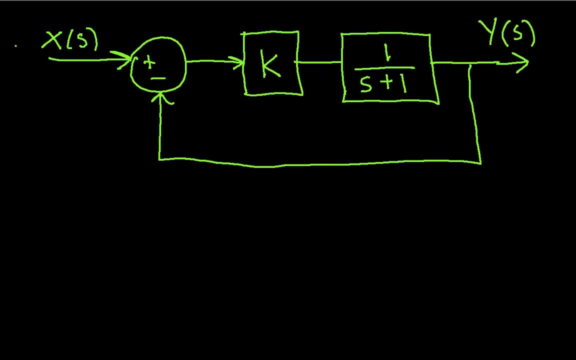 the Subtractor. So this is the error. This is the input to the system. Okay, So by looking at this, hopefully you can see that my plant has a transfer function of 1 over s plus 1.. The controller has a transfer function of just the gain k. 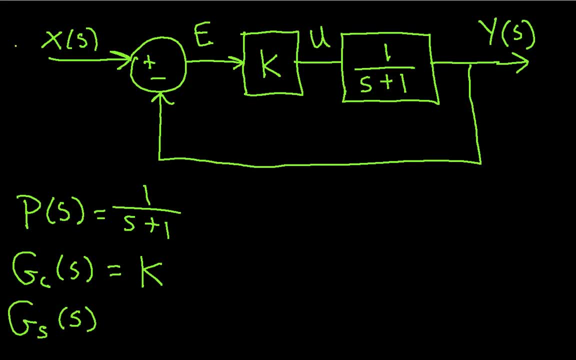 And the sensor transfer function- since I have the output y directly fed back into the error- just has a transfer function of 1.. Okay, With these values, the overall transfer function of this system. h Is equal to the overall number. 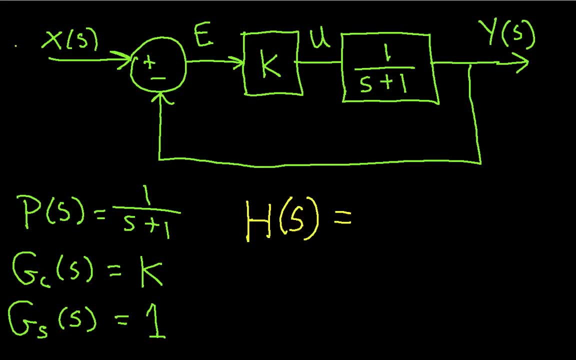 Let's see p of s, which is 1 over s plus 1, times gc of s, which is k over 1, plus p of s, which is 1 over s plus 1, gc of s, which is k, and g sub s of s, which is 1, okay. 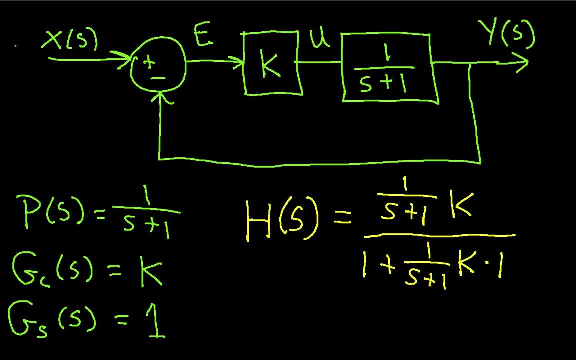 So, to make this a little more straightforward, I will assume that everybody's okay with just multiplying by 1, and I'll multiply the top and bottom of this fraction by s plus 1.. And when I do that, I get that this s plus 1 cancels this s plus 1,. 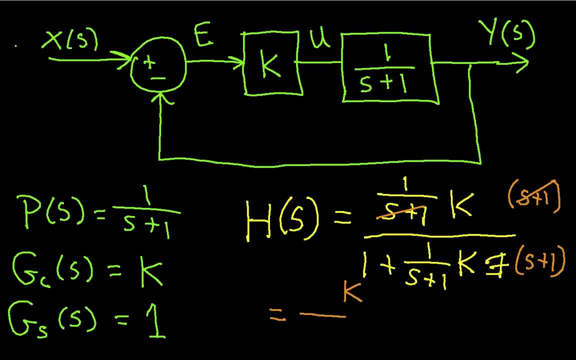 so I'm left with just k. Okay, Okay. So in the numerator this s plus 1, this one right here cancels this s plus 1, and this s plus 1 is multiplied by this 1 out here, so I get then s plus 1 plus k. 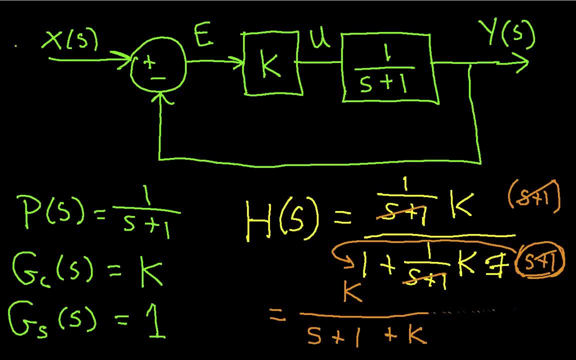 I'll tidy up this fraction here just a little bit. So basically, what we have then is the transfer function is 1 over s plus 1 plus k. Okay, I'm sorry, k over s plus 1 plus k. 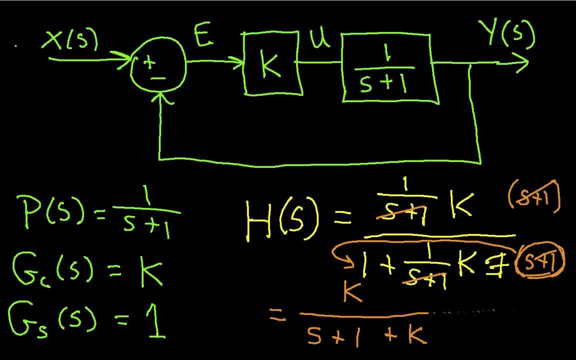 Okay, so that's the transfer function from output to input. You can see if we now draw a pole, zero plot of this transfer function: this is the imaginary axis and this is the real axis. so this is imaginary and real. The pole that this. this is imaginary and this is real. so this is real. 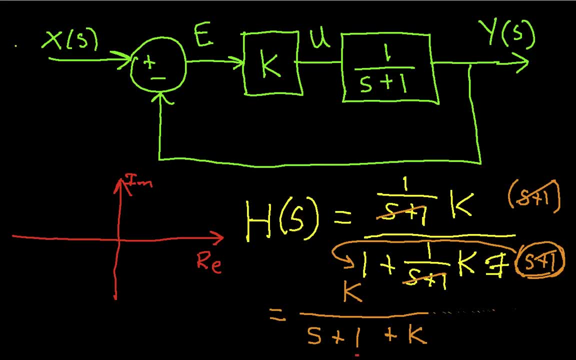 this transfer function has a single pole, given by this 1 plus k. here- And you'll remember the form of these expressions for poles is s minus the pole. So s plus 1 plus k means that there's a pole over here at a value of minus 1 minus k. 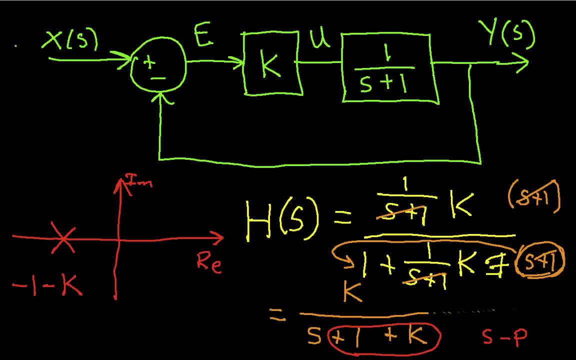 Okay, so you can see that I've taken my original system, which had a pole at minus 1, and I've moved that pole to the left. assuming that k is positive, I've moved that pole to the left. What this implies, then, is that my original system had a transfer function. 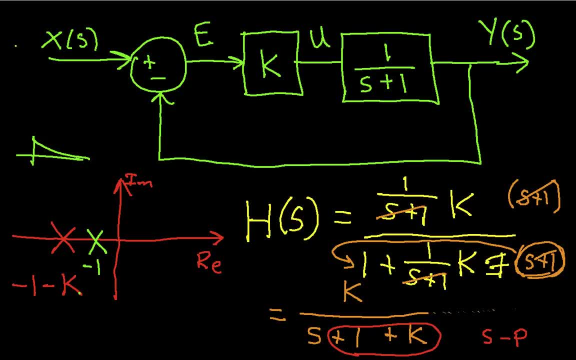 or an impulse response that looked something like: With the feedback, I'm able to make the impulse response look something like this. In other words, by moving this pole to the left, I've decreased the time that it takes for the system to respond to changes in the input. 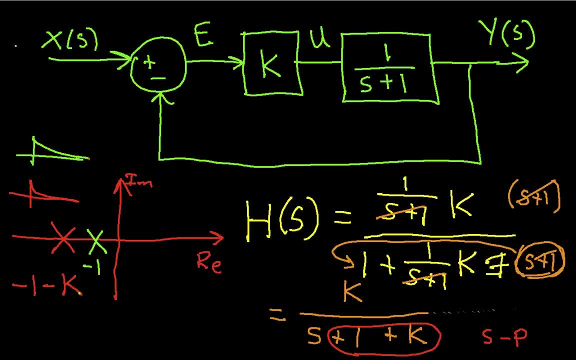 Okay, now again, that assumes that k is positive. What happens if k is negative? So we'll actually put here: this is k greater than 0.. If k is negative, what happens? What happens here? Well, if k is more negative than negative 1, I can actually move my pole out here. 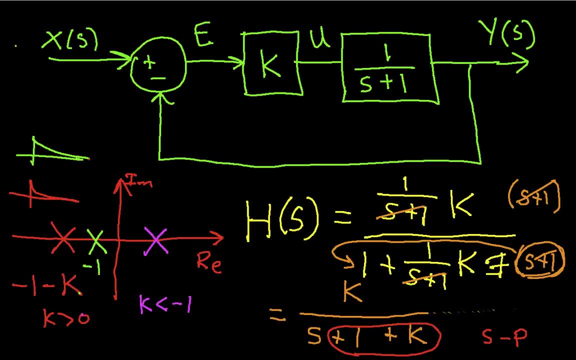 So if k is less than negative 1, I've moved my pole out here, and this corresponds to a transfer function that looks like this: So by having a negative gain, what I've actually done is I've moved my system to become unstable, which is typically a bad thing. 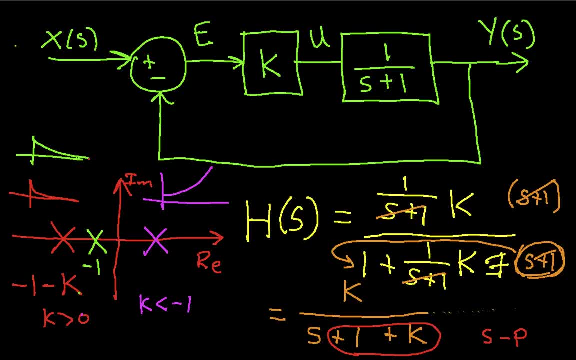 So this is probably the simplest example you can come up with of a feedback system, and you can observe how the gain changes the location of the single pole in the original system. Positive values of k make the pole move to the left. Negative values of k make the pole move to the right.